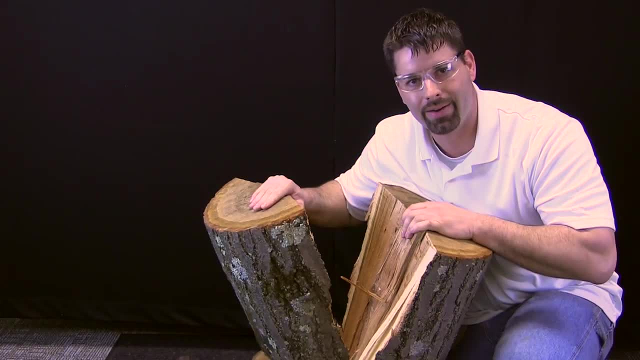 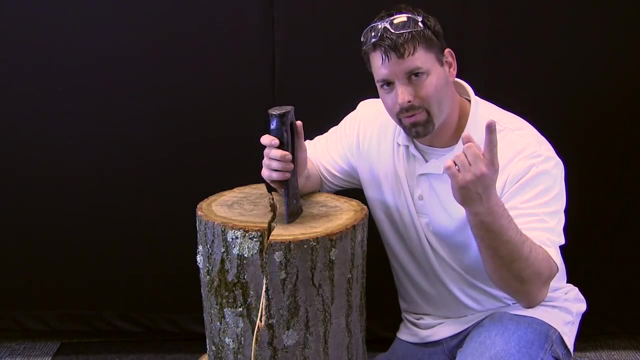 the wedge at work, But what we want to do now is take a close look at, really, how is this wedge working. To do that, we are going to go to the table with some other neat demonstrations Now to take a closer look at how a wedge actually 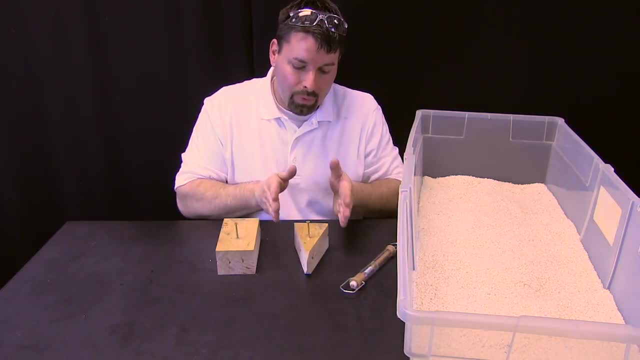 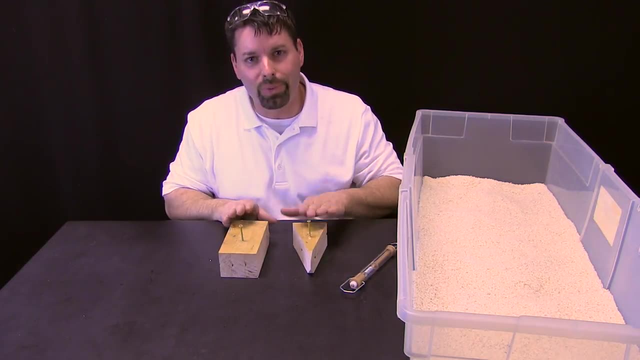 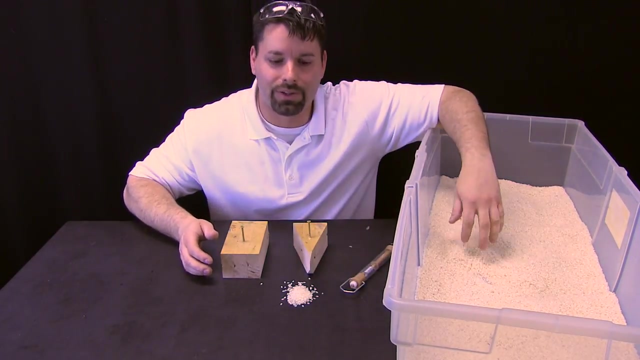 works. we need to do some measuring To do that. we have one block that is a wedge and another block that is not a wedge, And I want to see how much force it takes to move both of these blocks through some dry rice. All I have here is actually three big bags of 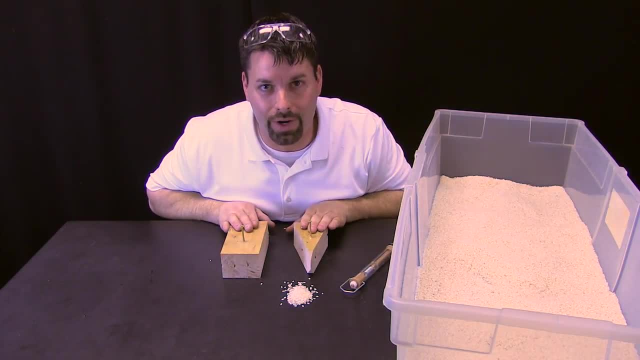 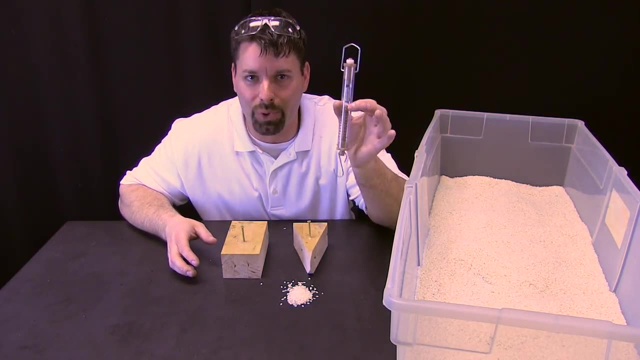 dry rice and we are going to try and move these blocks through that dry rice to see how much force it takes. How do we know how much force it takes? We are going to use our good old, trusty spring scale. So we have our block in our bin of rice and I want you to. 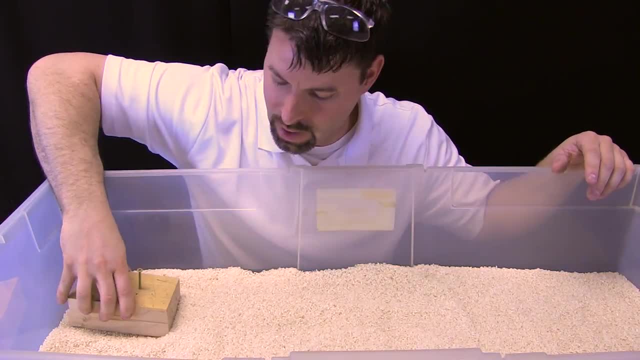 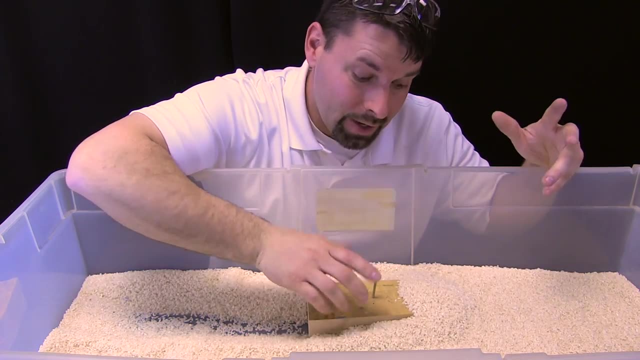 watch what happens to the rice when I push my block through the rice. As I push it through the rice, you can see the rice does not do a good job of separating It. all kind of bunches up in the front. Now let us see what kind of force that takes. 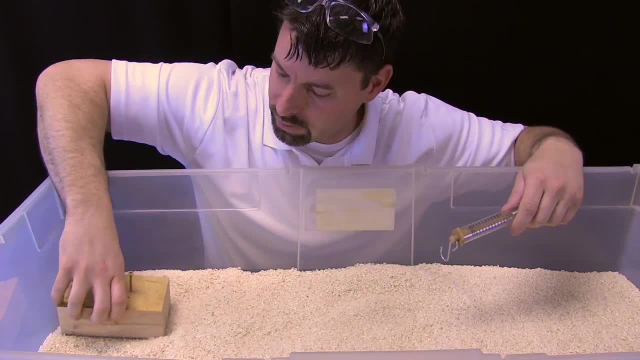 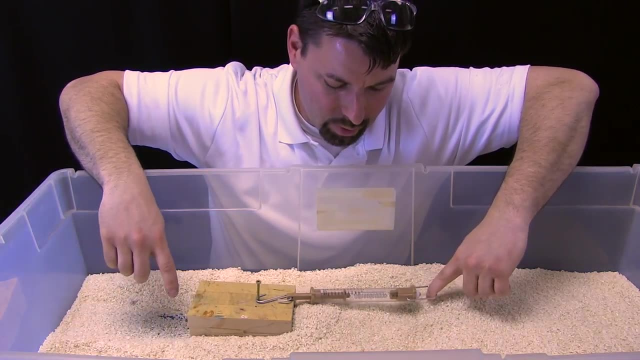 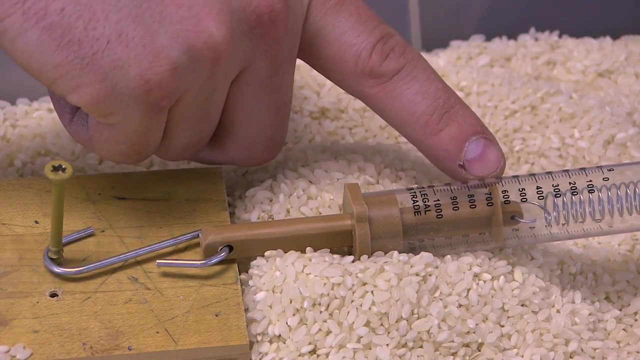 as we push the rice through. Here is a block through the rice. I will bring in my spring scale, put it on to my block and I will begin to pull. As I pull, you can see I am pulling about 600 grams with this. 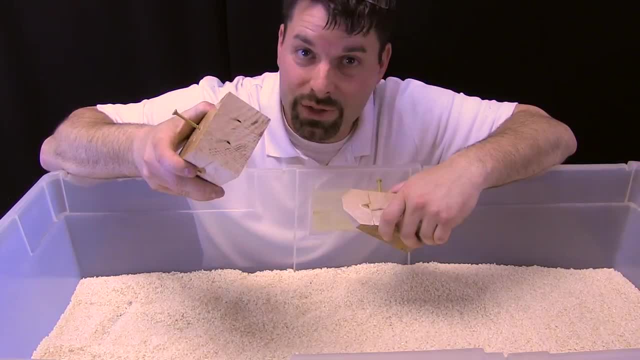 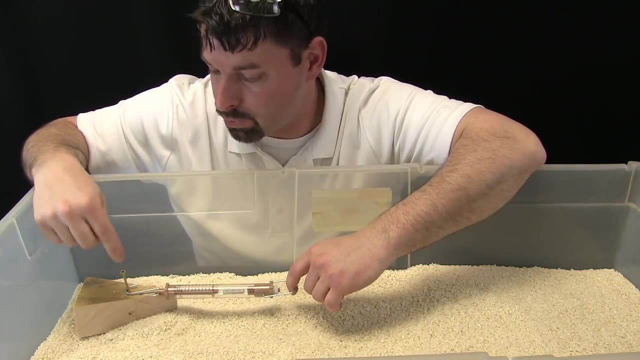 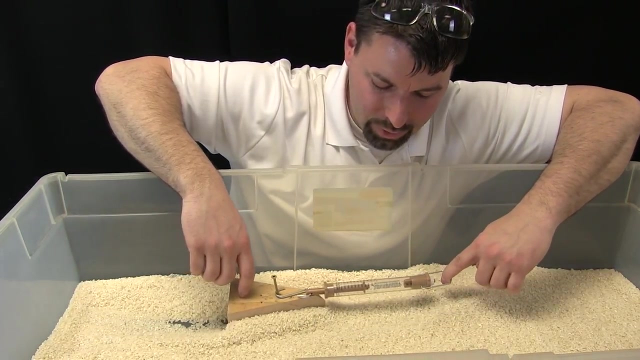 flat block. So we have seen what our flat block can do. Let us see what our wedge does as it travels through the rice. So let us start to pull this wedge through the rice. Take a close look, Take a close look at the spring scale. as I pull, I start to pull and it is pulling. 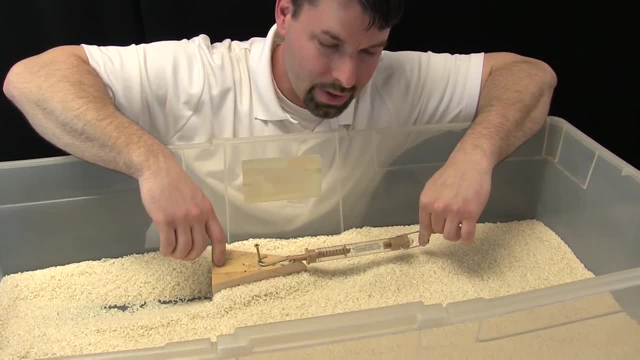 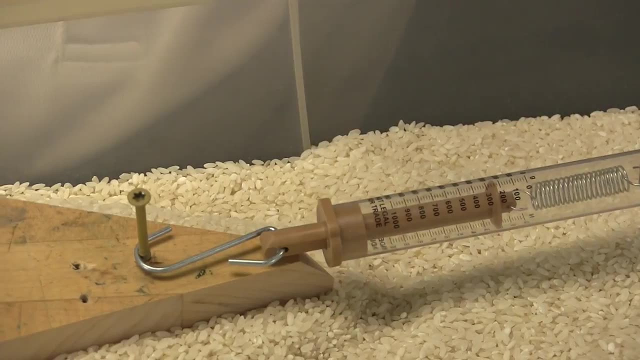 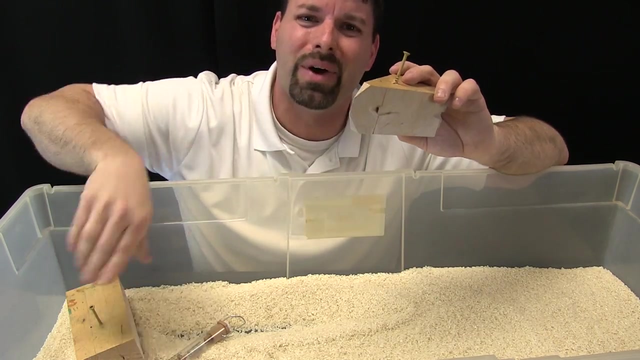 about 300 grams. I am going to stop right there so you can see. We will zoom in. It is just that: 300 grams. You can see it moves as soon as I tug. So this flat block took about 600 grams of force to move it through the rice, but this wedge took about half that. 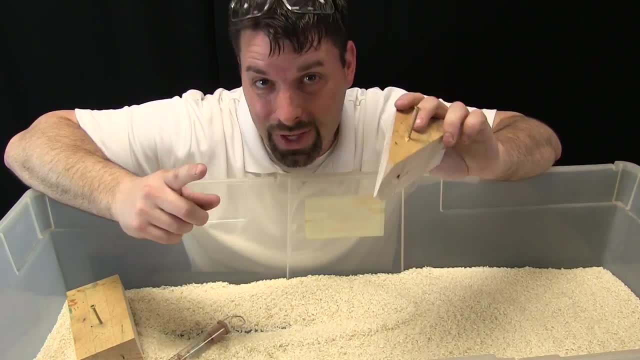 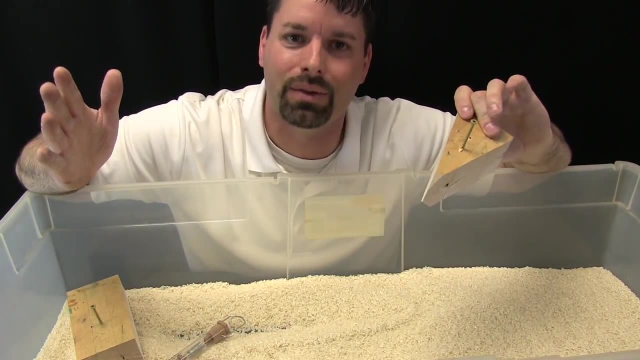 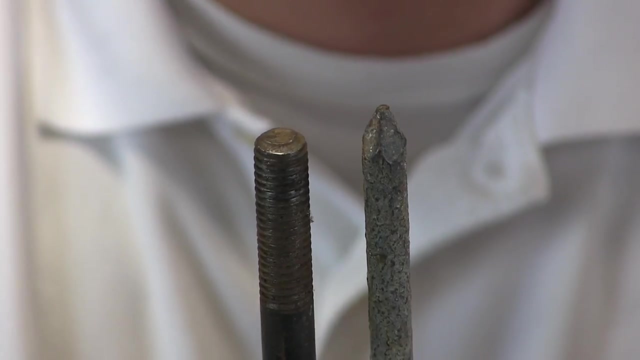 Only 300 grams of force to move this wedge through the rice. I would say that, looking at our data, The wedge really does make our job easier of separating things and moving things apart. Wedges are at work all around us. Take a look at this: These two pieces of metal are actually.